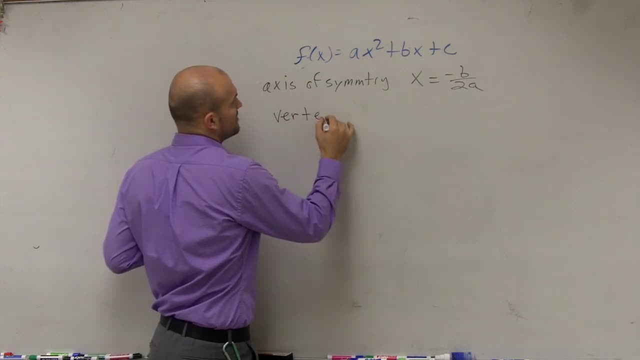 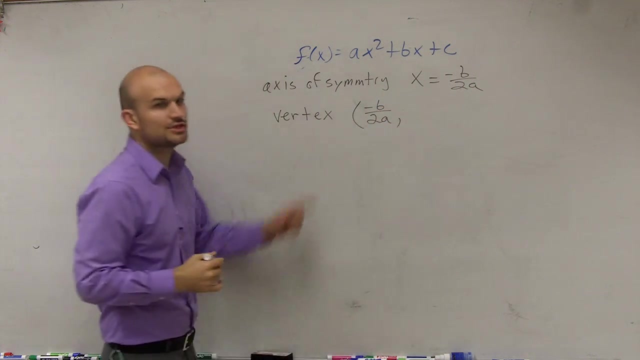 Then we also said we could find the vertex. Now, how did we find the vertex? Well, remember, this was your x coordinate of your vertex. Then what you had to do to find the y coordinate is: you'd plug this value into your function. 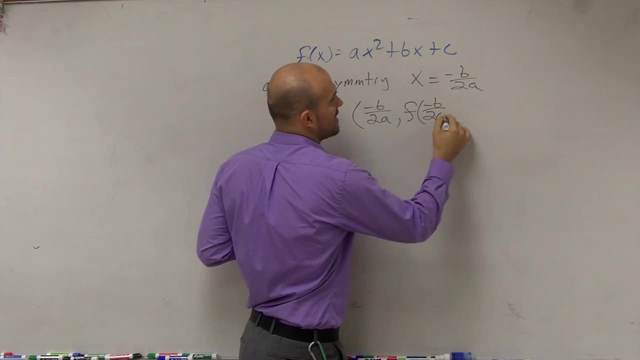 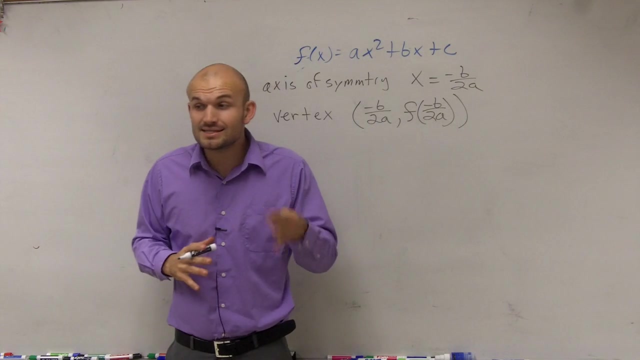 So the way we represent that was using function notation of f of 2a. So that was how you find your vertex. Now, the only other thing that we- well, not the only other thing, The next thing we kind of talked about, this is all review. 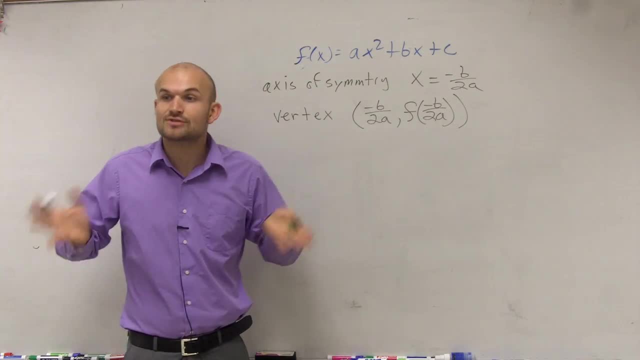 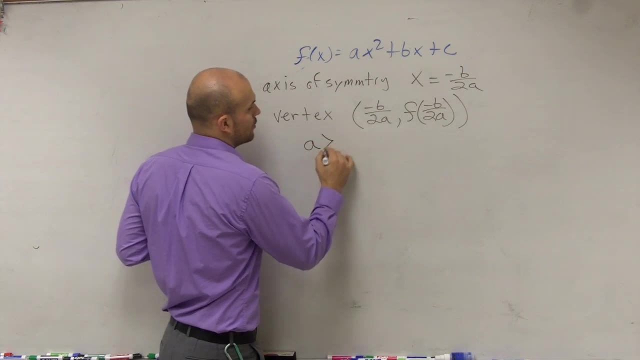 The next thing we talked about was how to find if it's a max or a minimum, right, Is your vertex a maximum or minimum? So to do that we looked at the value of a. If a was greater than 0, then we said our vertex was a minimum point right. 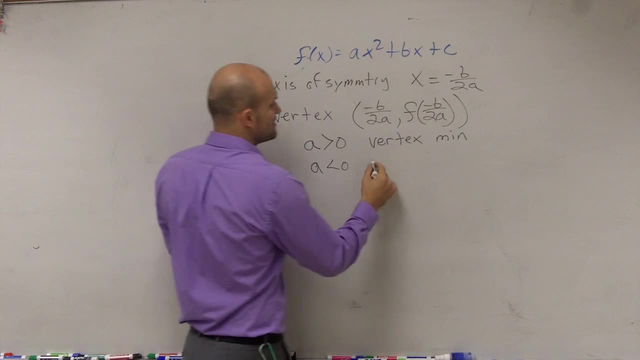 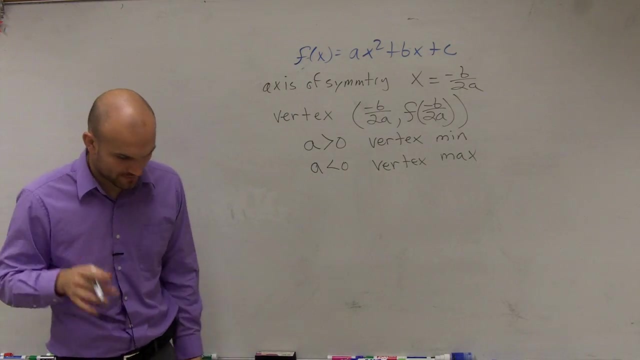 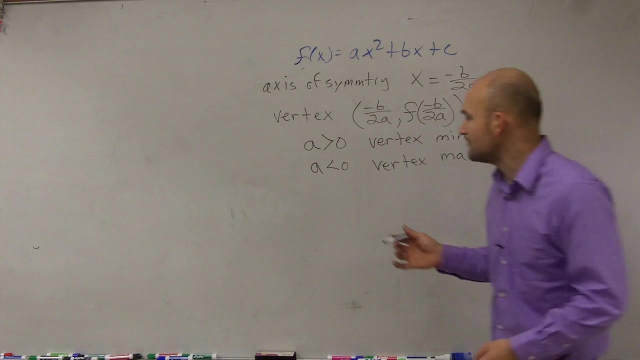 Then we said if a was less than 0, then we said our vertex was a maximum point, correct, Correct, Okay. Then the last thing we talked about was how to find the x and y intercepts. So to find the x intercept? no, I'm sorry, let's do y intercept first. 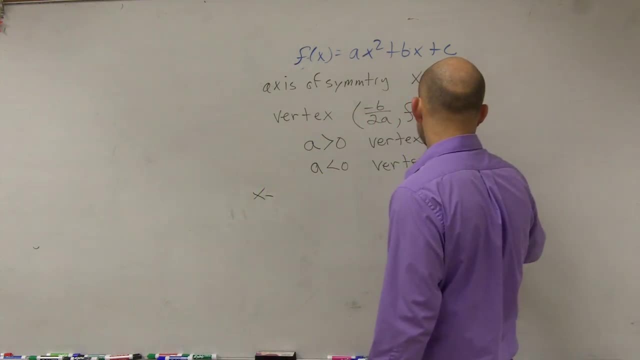 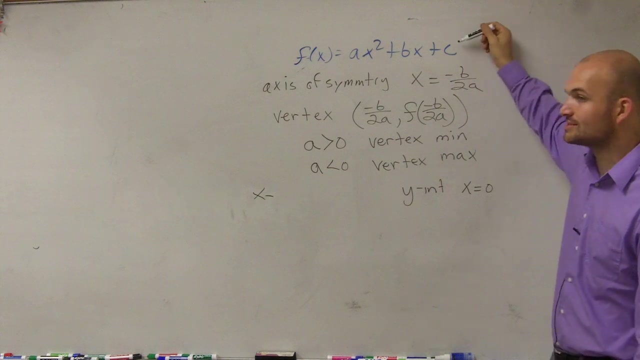 To find the y intercept. all we simply did was say, put x equal to 0. So what we did is we put 0 in for x and what we noticed was the x intercepts usually are constant, right, Because 0, you're multiplying. anytime you're multiplying, you're going to get rid of your a and b. 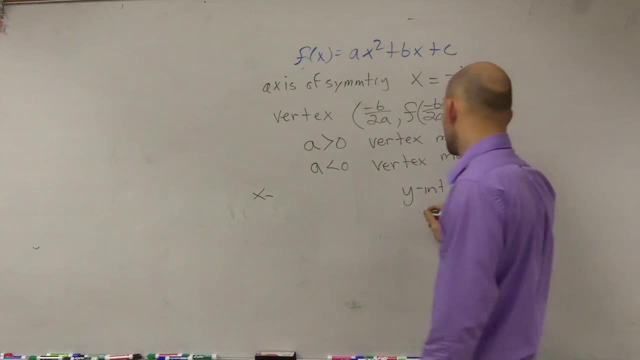 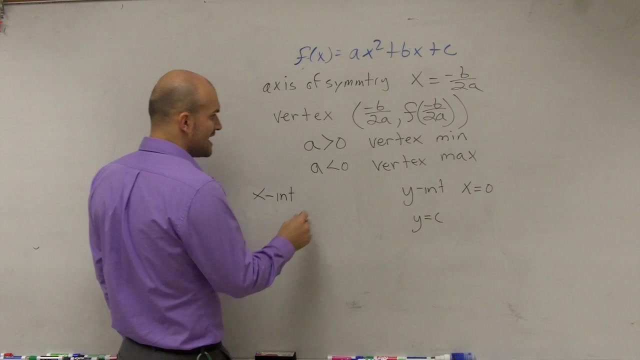 So your y intercept was always what c was equal to. So we'd always say kind of y equals c. Then we said: find the x intercepts. To find the x intercepts we said y equals 0, or in function notation you could say f of x equals 0. 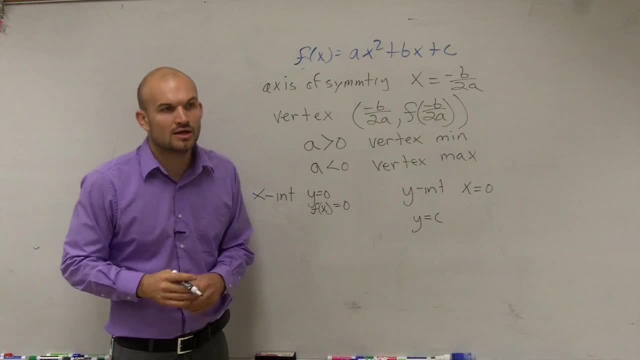 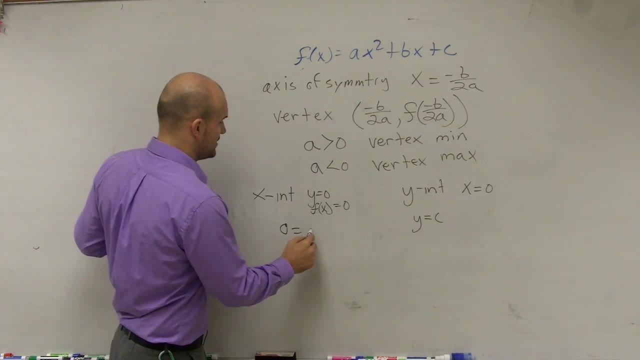 All right, it really kind of means the same. you know thing, f of x is going to be your dependent variable. So now remember when we had something like this, we'd say: 0 equals ax, So our x is going to be x squared plus bx plus c. 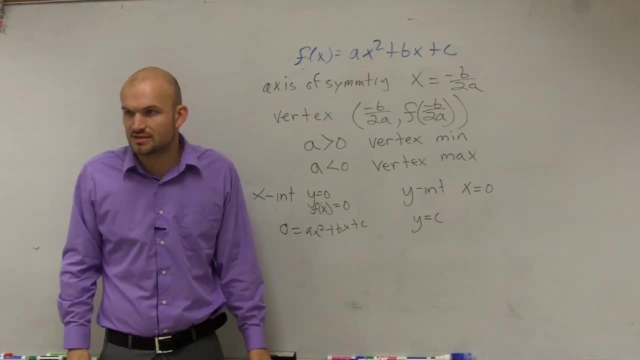 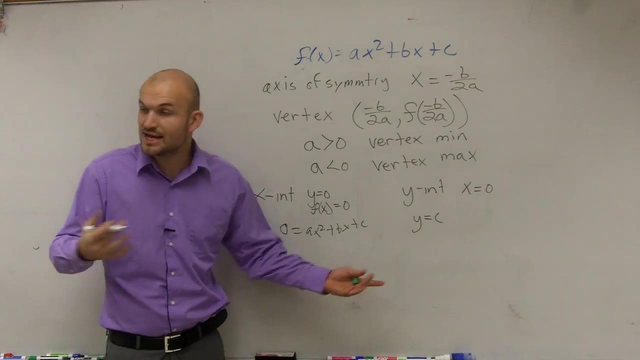 What was the only way we could find the value, or what was the way that we learned to find the value of x's on your previous test, You had to do what Well that was? to graph it right. we graphed it with tables. 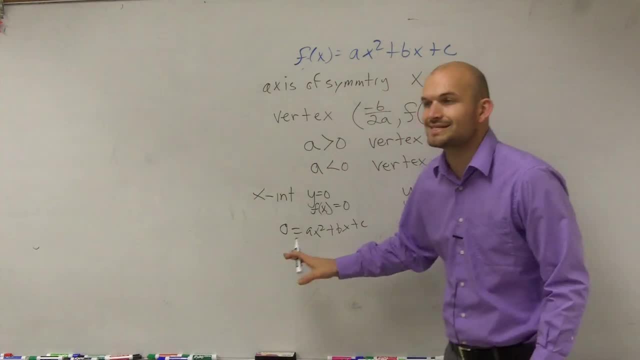 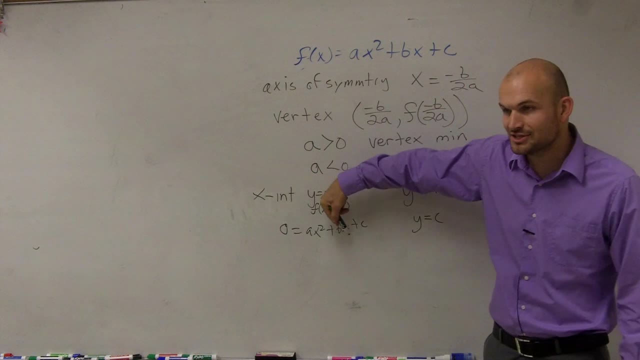 And, yes, you could have found the x intercepts with the tables. but we also learned another way to find just the x intercepts as well. Rhymes with factoring, Factoring- right, We learned how to factor it, Factoring and tracking. 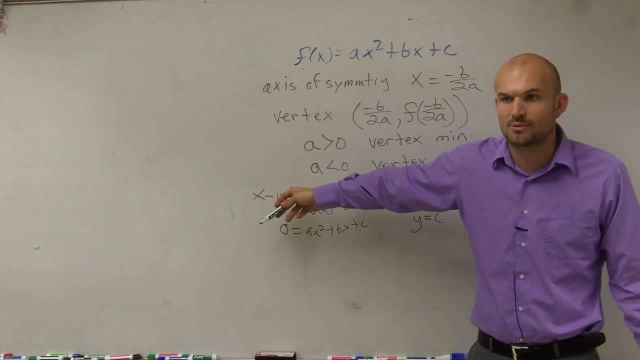 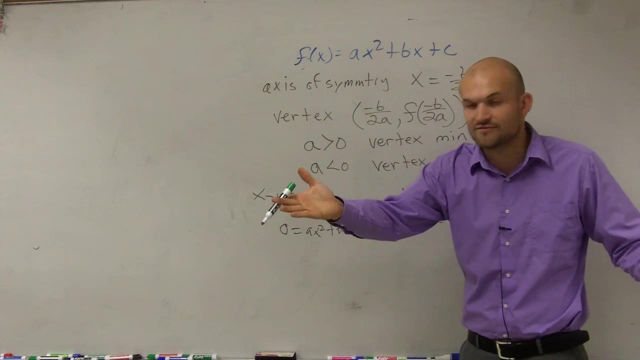 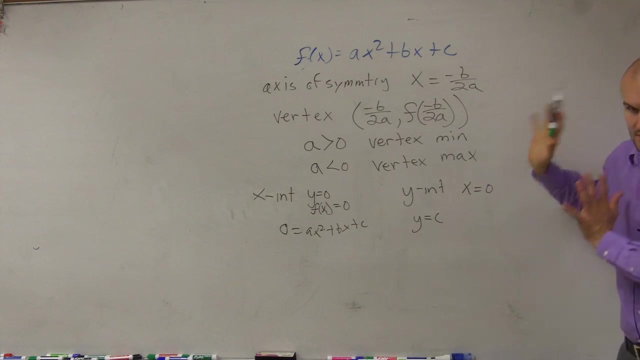 Okay it. and then we solved by using the zero product properties. everybody remember that, right. but then there was times when we couldn't factor it and we had to rely on our table of values right to find the x-intercept. so they remember that. okay, that is a review of that. okay, that's when you have standard form. okay, there's. 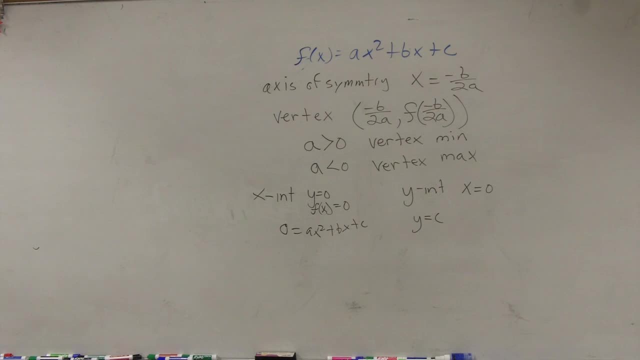 your review. okay, so what are we talking about? 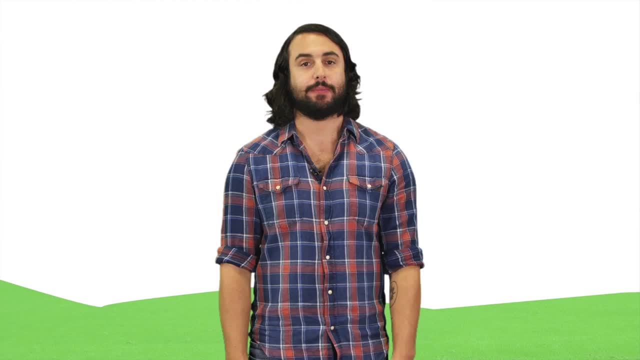 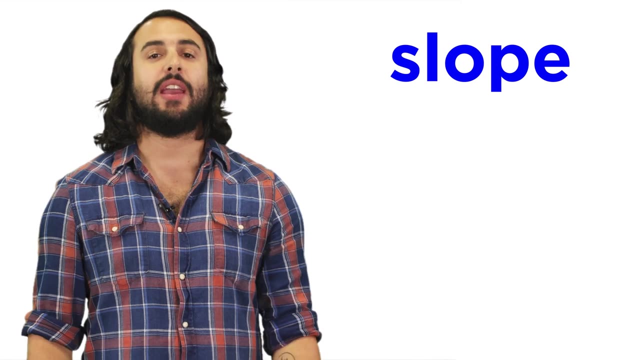 Professor Dave, again let's talk about slopes and intercepts In math. when we use the word slope, it doesn't mean we are going to hit the slopes, although there is some similarity between the downward slope of a mountain and the meaning of this. 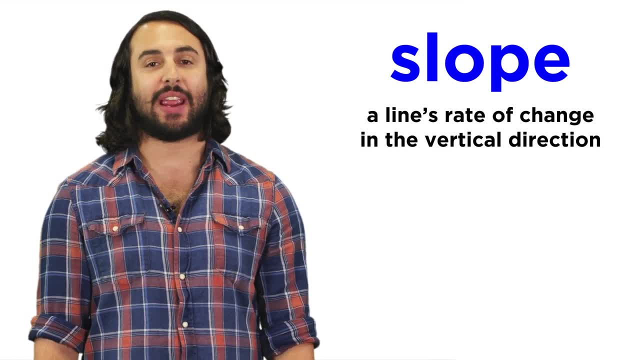 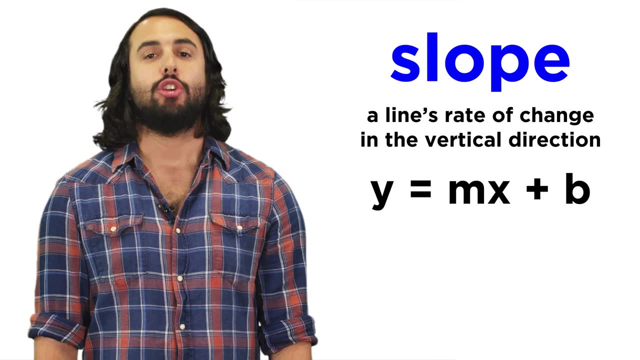 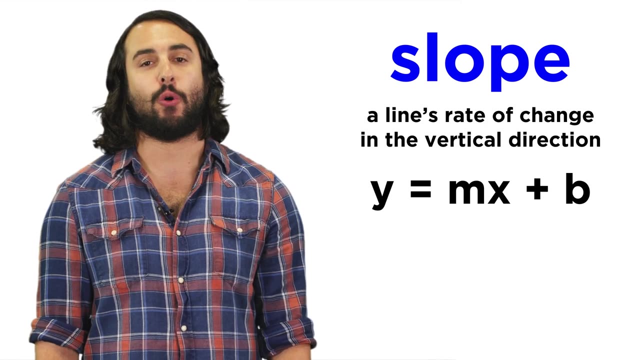 word. in math It means a line's rate of change in the vertical direction, which can be shallow or steep, just like a mountain. To understand how the slope of a line relates to the equation of the line, let's introduce a common form for linear equations: y equals mx plus b. 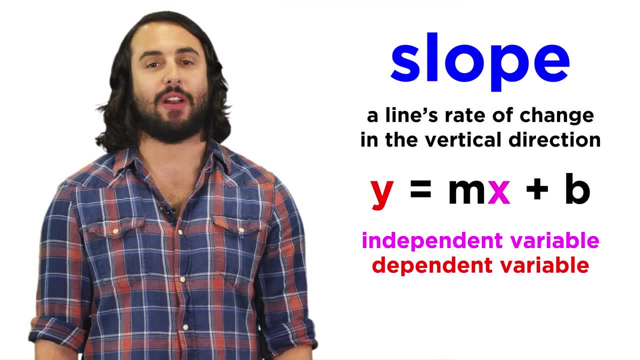 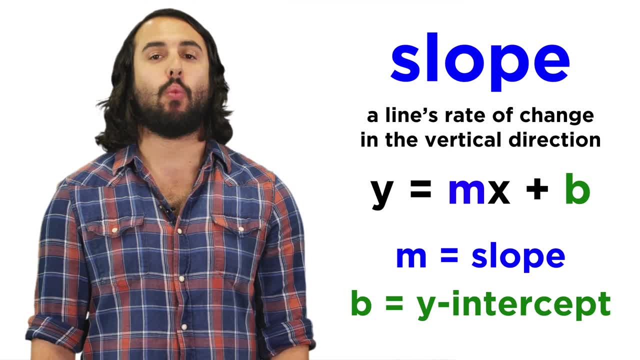 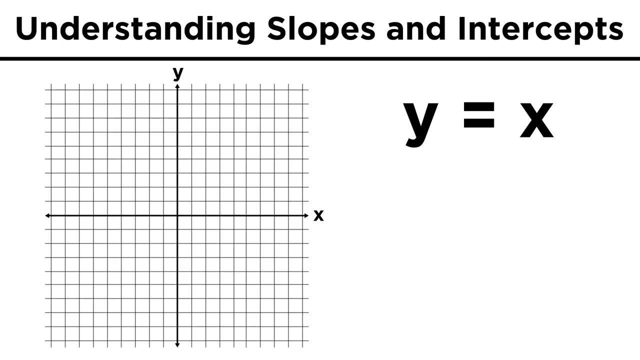